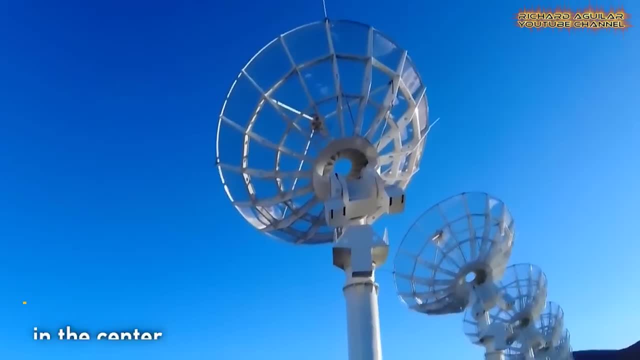 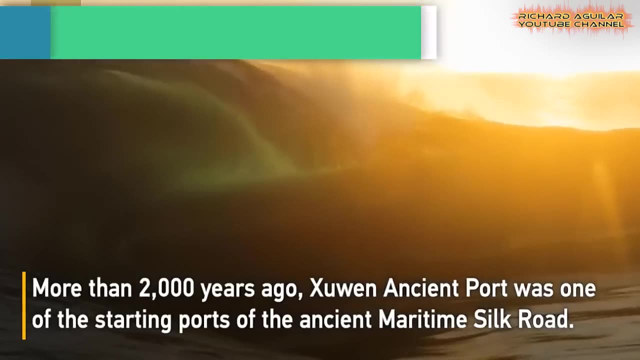 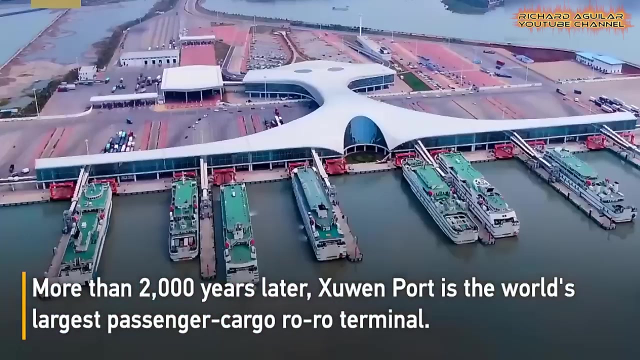 This significant achievement marks a milestone in China's advancements in radio astronomy and space science research. Chinese President Xi Jinping recently visited Guangdong Province and toured Sichuan Port in Zhenjiang City to gain insights into the region's transportation infrastructure improvements and the two-way development of Guangdong and Hainan Provinces. 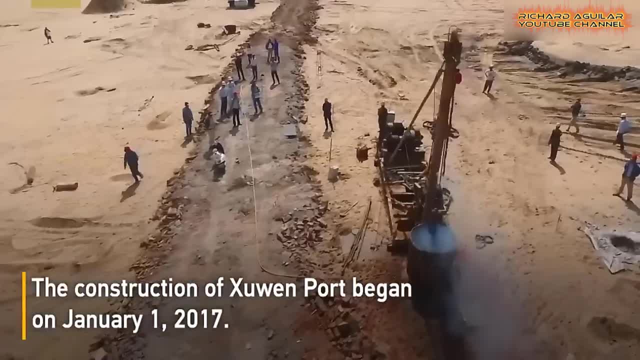 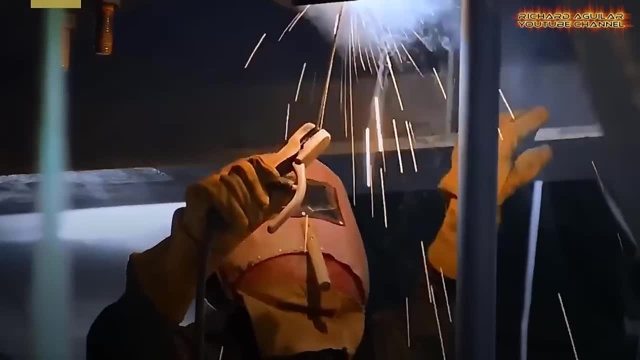 Xi Jinping and Li Center of Defense in China are two of the country's largest shippingрcunenses. Sichuan Port, located at the southernmost tip of the mainland, is the world's largest passenger cargo RRO terminal and plays a crucial role in facilitating regional trade and economic growth. 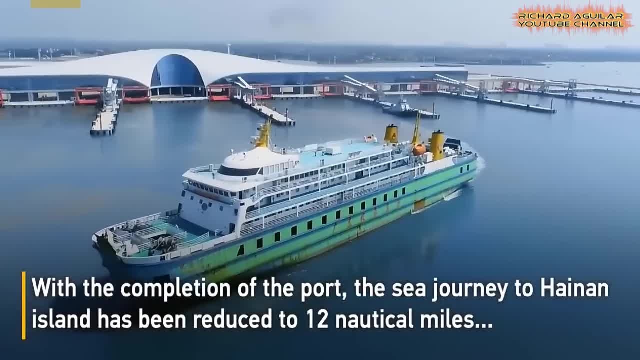 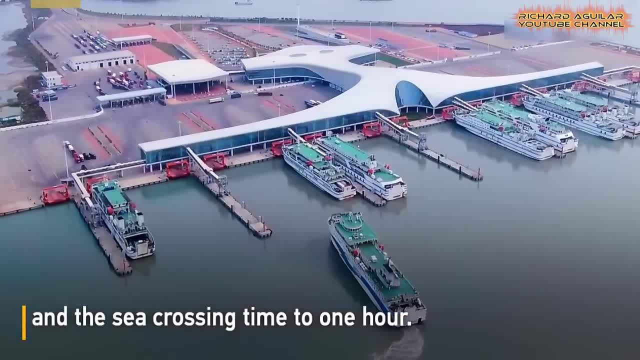 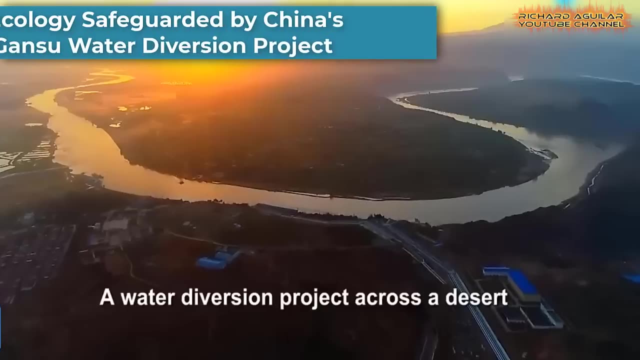 President Xi's visit underscores the Chinese government's commitment to advancing transportation infrastructure and promoting regional development in support of regional development and promoting regional development in support of economic growth and prosperity. For over 20 years, a pioneering water diversion project has been making a significant impact. 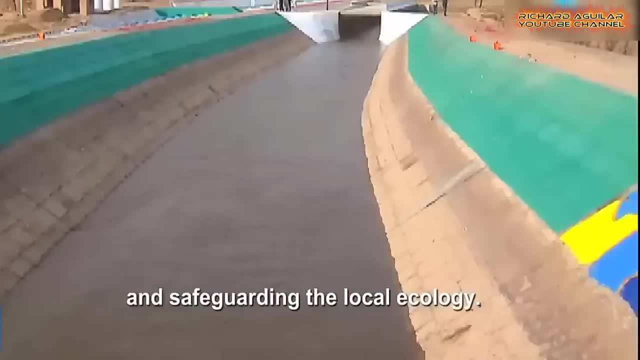 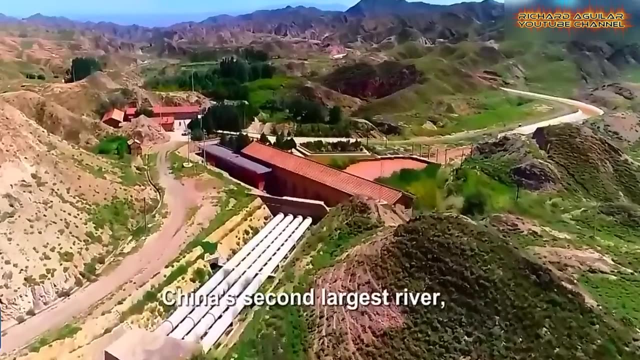 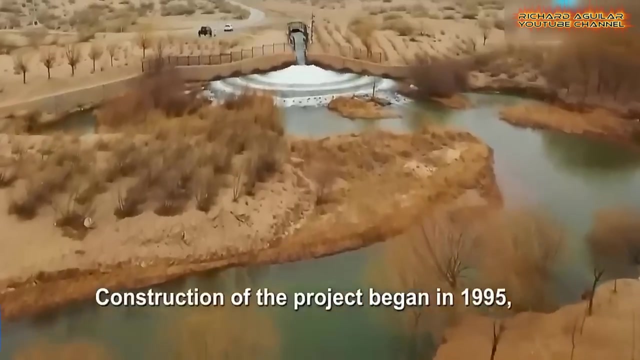 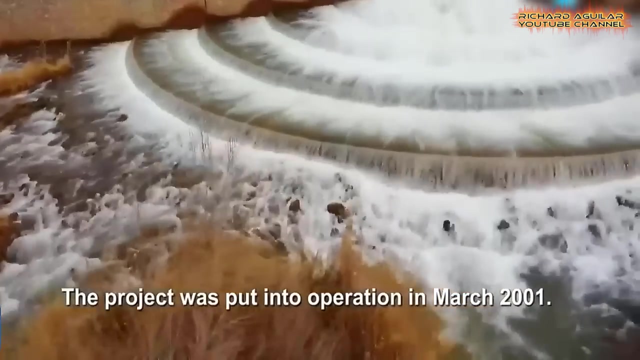 in northwest China's Gansu Province. This ambitious undertaking has successfully brought water to a desert region, benefiting local residents and protecting the local ecology. The water diversion project has involved channeling water from nearby sources to the arid regions of Gansu Province, which has long struggled with water scarcity. 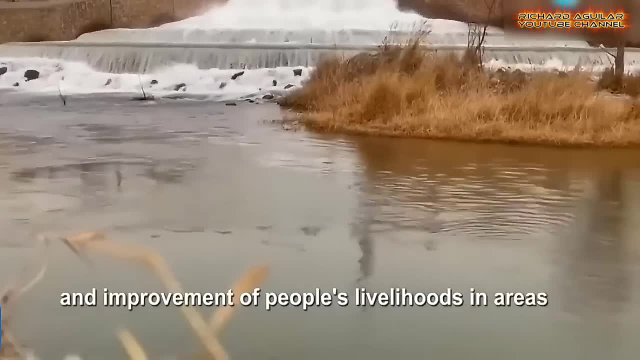 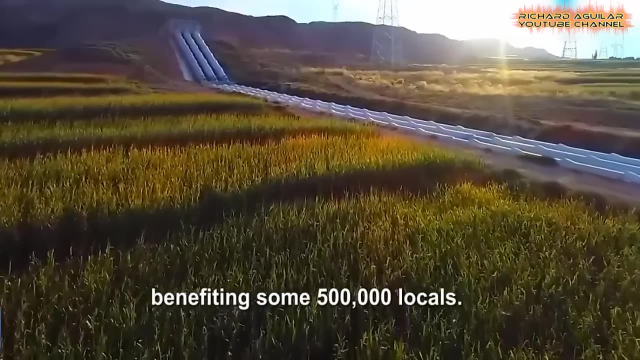 Through an intricate network of canals and pipelines, the project has provided much-needed water for drinking irrigation and other daily needs of local communities. This has enabled the development of agriculture, livestock farming and human settlements, improving the livelihoods of the residents and living in the area. 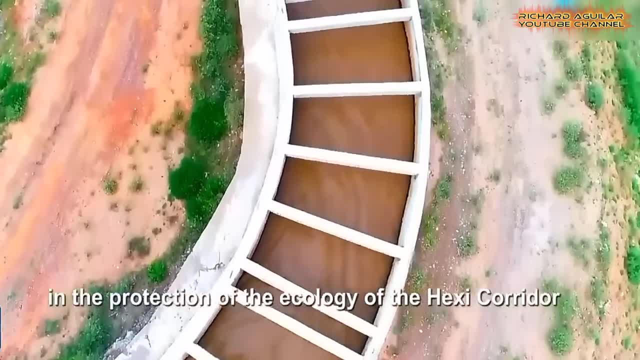 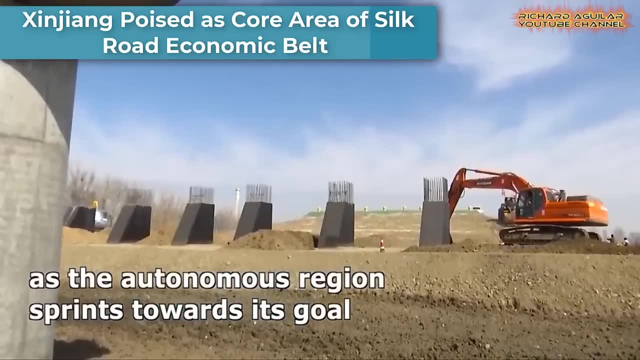 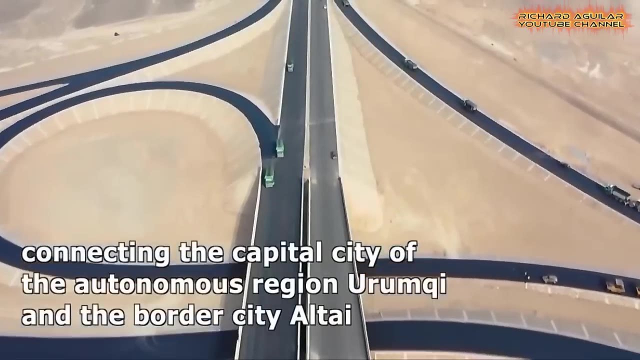 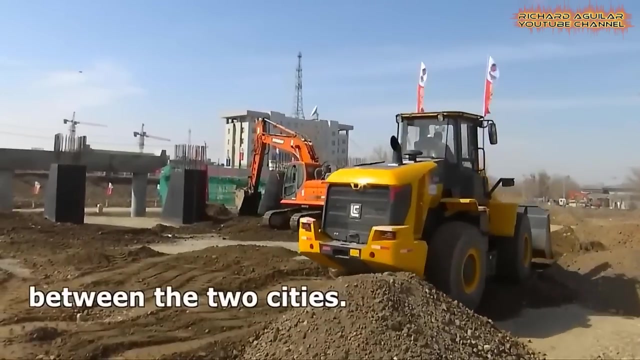 This is to provide a range of development opportunities for the local population and to ensure their prosperity. withoutействit is asking for another project. This is a big rescue project for the people who are living in poor neighborhoods, with many of them looking to adapt to the water issue in the region. 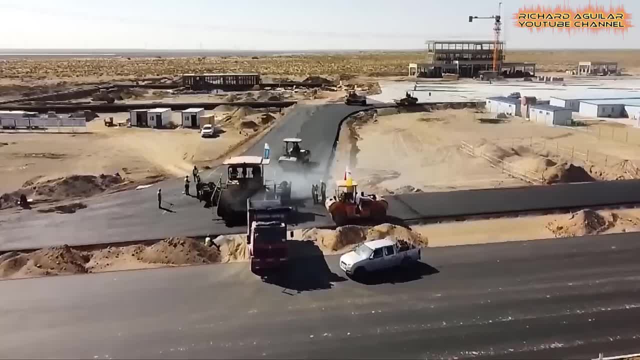 This project has been part of the project team's relatively numerous projects since the initial development, although a few of them have been lost to water this year. The first project was launched last year and is now in deployment. The project that included the central public station is currently under construction. 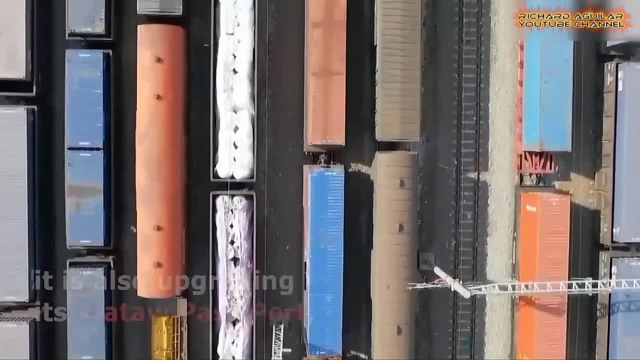 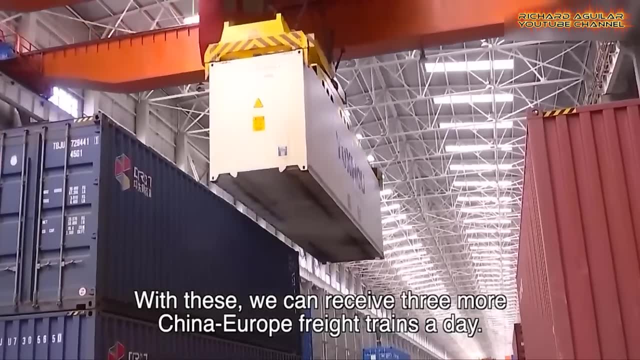 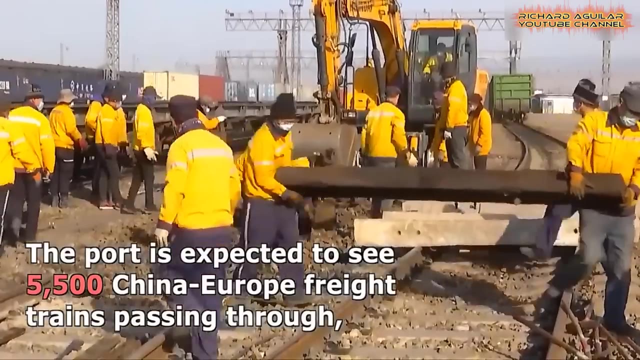 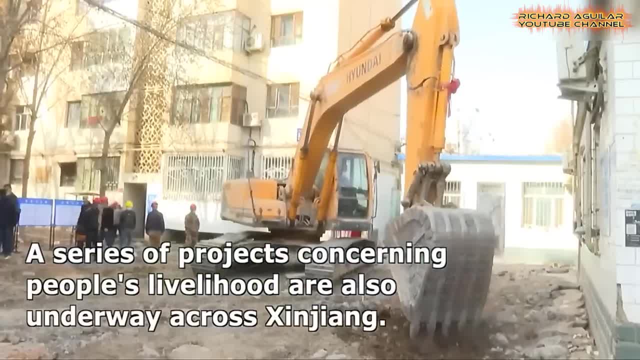 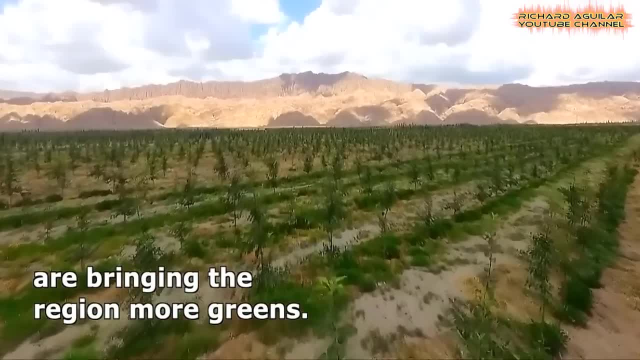 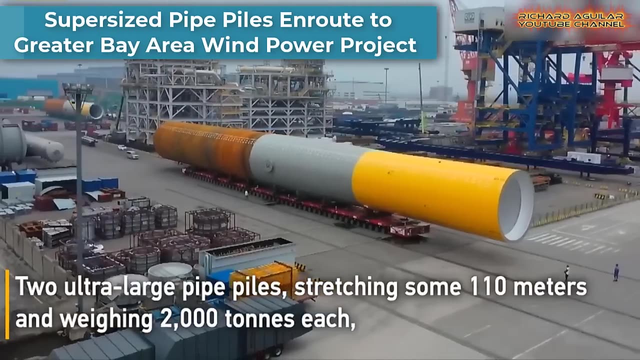 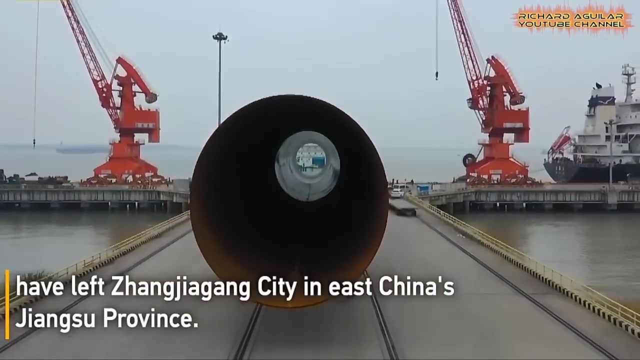 completed on time. All the 56 road projects across Xinjiang, which halted due to the COVID-19 epidemic, have resumed construction. China's ambitious wind power project in the Guangdong-Hong Kong-Macao Greater Bay Area has taken a significant step forward as two supersized pipe piles each weighing a staggering 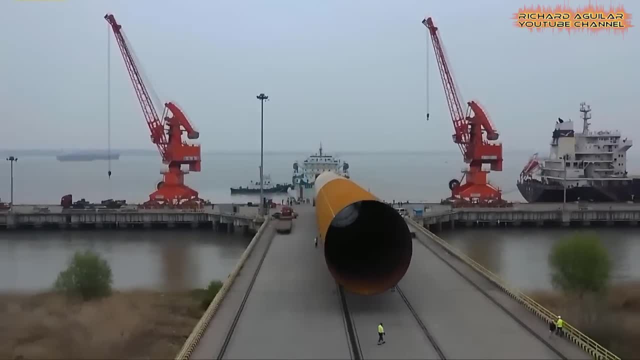 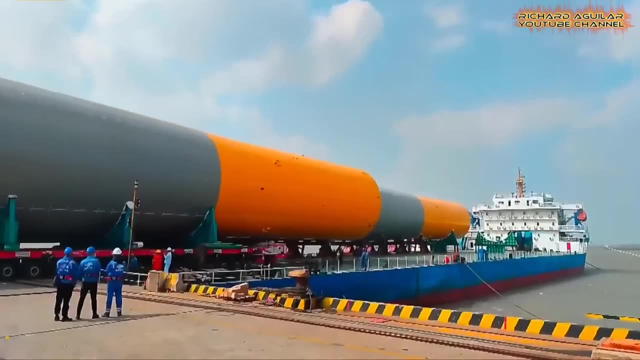 2,000 tons and stretching over 110 meters, have been transported from Zhangjiagang City in Jiangsu Province to Huizhou City in Guangdong Province. The enormous pipe piles are critical components of the wind power project. The project aims to harness the region's abundant wind resources and promote clean 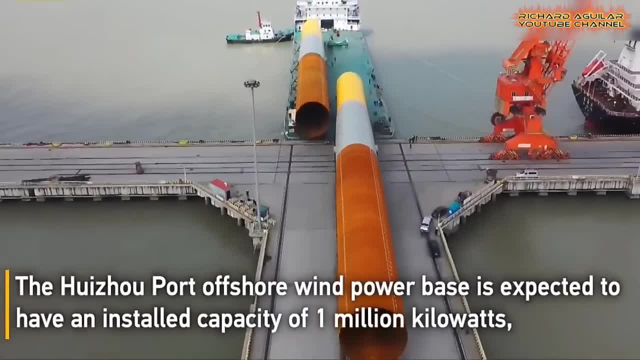 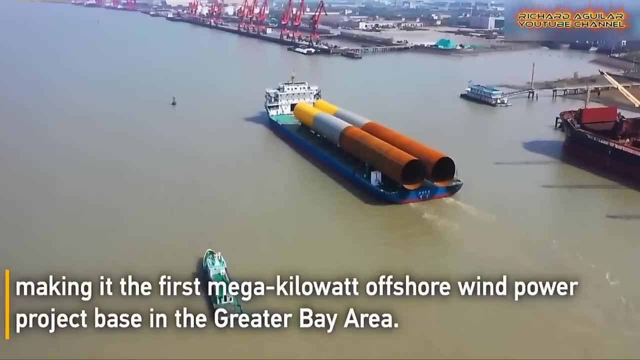 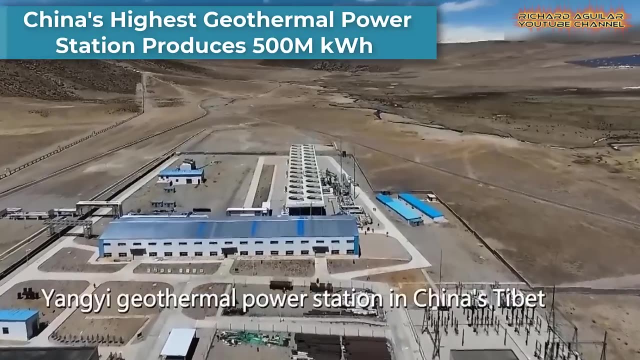 and renewable energy generation. The successful transportation of these ultra-large pipe piles highlights China's commitment to investing in sustainable energy infrastructure and promoting green development in the Greater Bay Area. China's Yangyi Geothermal Power Station, located in Tibet and recognized as the country's highest-altitude geothermal power station has been a remarkable success since its inception in 2018.. It has already generated over 500 million kilowatt-hours of electricity, showcasing the immense potential of geothermal energy in China's renewable energy landscape. 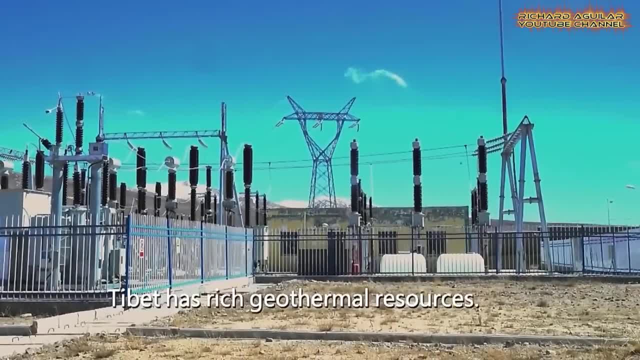 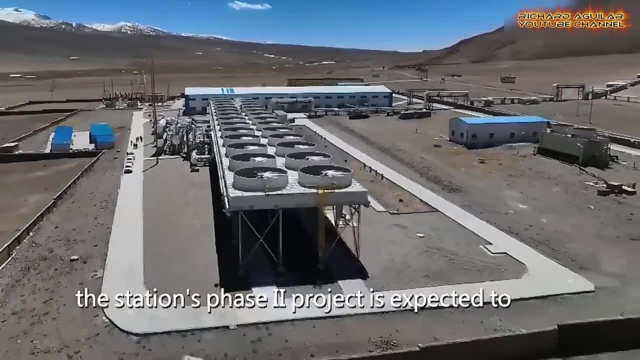 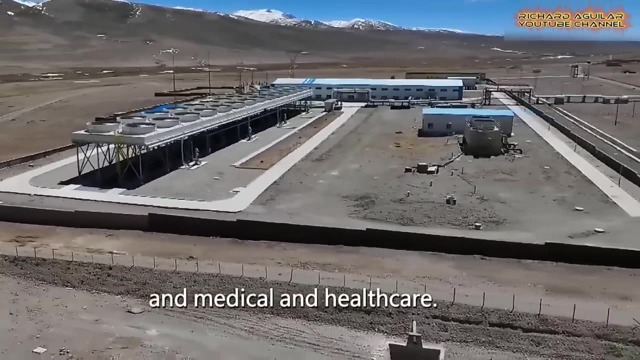 The Yangyi Geothermal Power Station has harnessed the natural heat of the country's energy production to generate clean and sustainable electricity, reducing greenhouse gas emissions and contributing to the country's efforts towards combating climate change. China, the world's most populous country and one of the fastest-growing economies, has 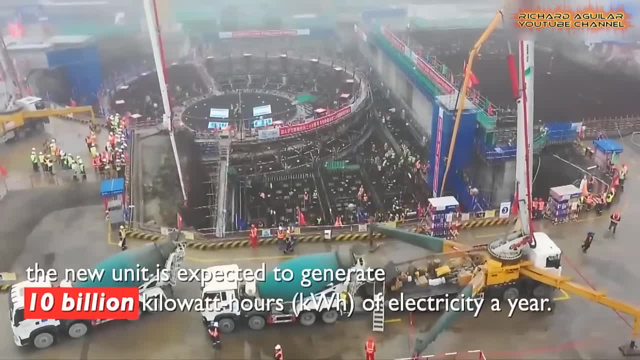 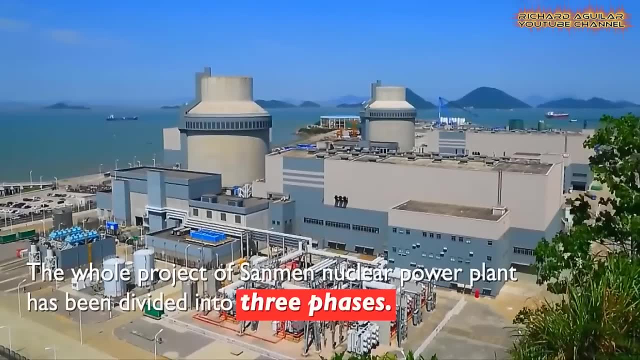 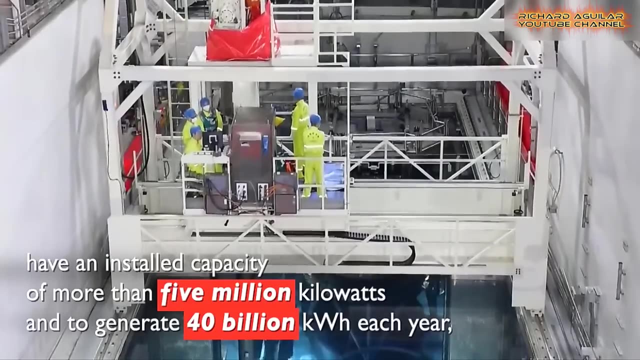 embarked on a new milestone in its pursuit of clean and reliable energy sources. In an effort to meet its increasing energy demands, China has begun construction on a state-of-the-art nuclear power plant, located in Taizhou city of east China's Zhejiang province. 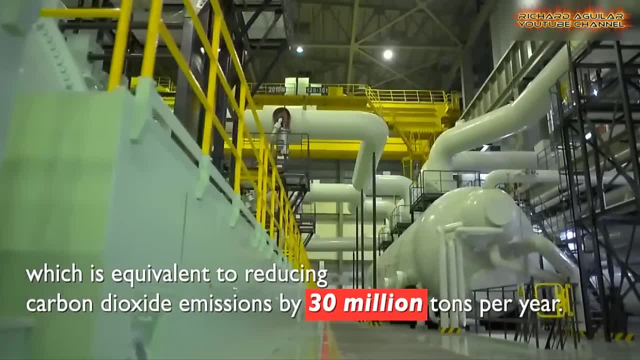 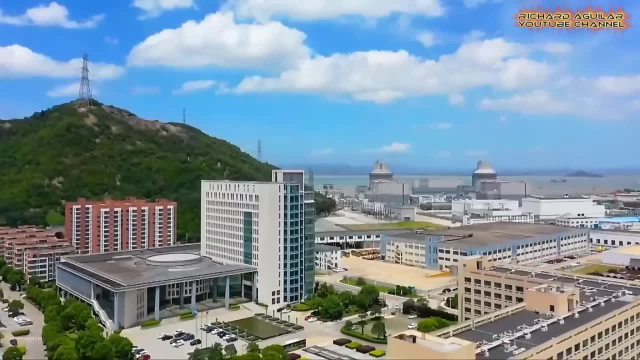 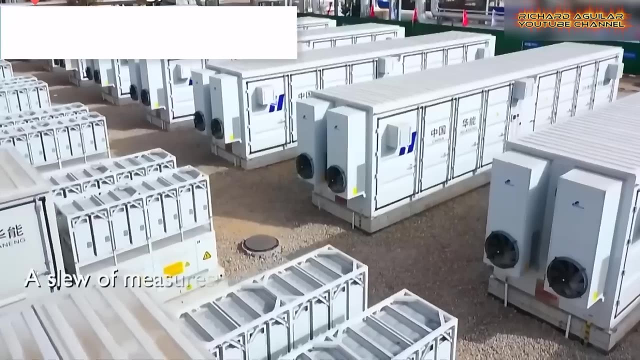 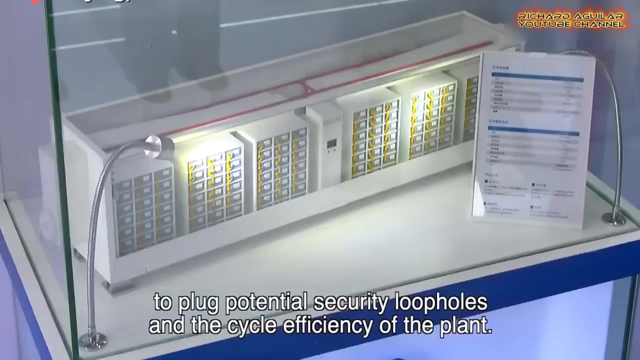 The new nuclear unit is expected to generate 10 billion kilowatt-hours of electricity a year. A slew of measures have been adopted to turbocharge the energy storage industry in China, which insiders believe will spur rapid growth of the industry in the country. 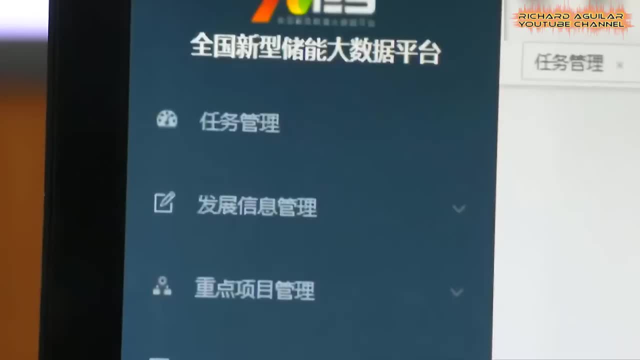 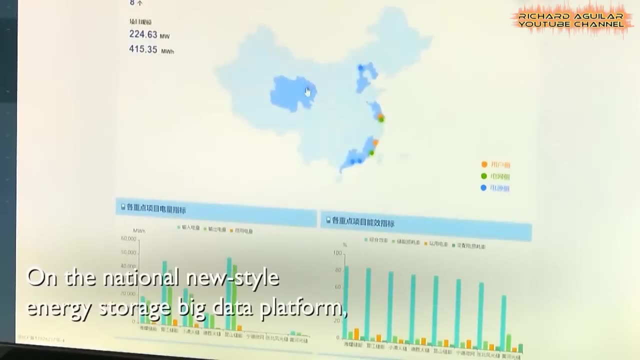 In Jinan City, East China's Shandong Province, a 100-megawatt lithium-ion battery storage power station has been in operation for one year, which uses a digital technology, innovation and intelligence system to control each battery cluster precisely Compared with traditional. 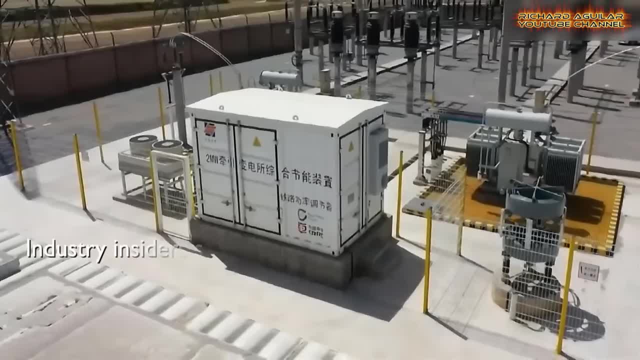 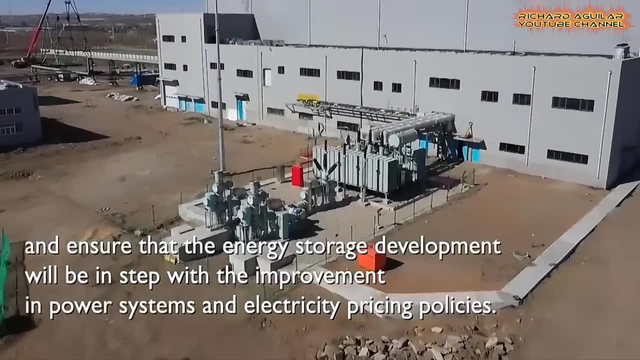 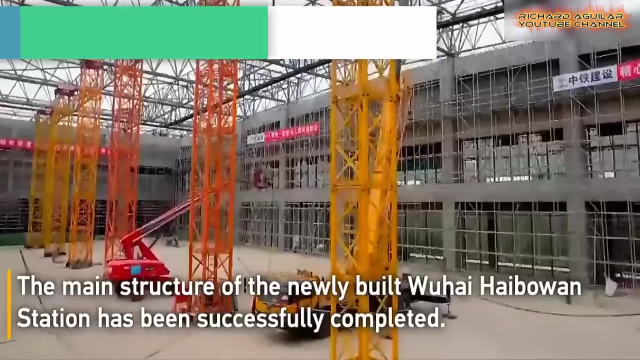 energy storage power stations. this plant's available capacity marks an increase of 7.5%, which helps reduce the initial investment effectively. A significant milestone has been achieved in China's Inner Mongolia Autonomous Region with the successful completion of the main structure of the Wuhai-Heibewan Station. 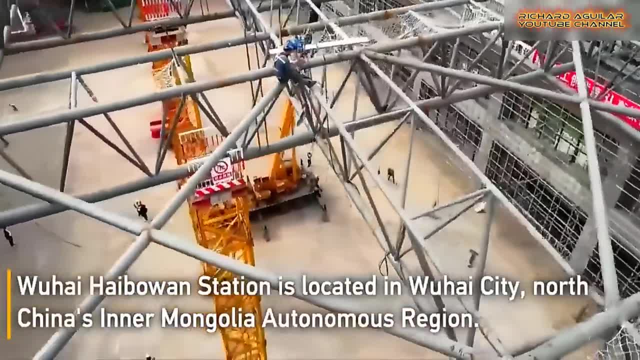 This newly built station is part of the Baotou-Yinchuan High-Speed Railway and it is the largest station in the entire project. Located in Wuhai City, the Wuhai-Heibewan Station is the largest station in the entire project. 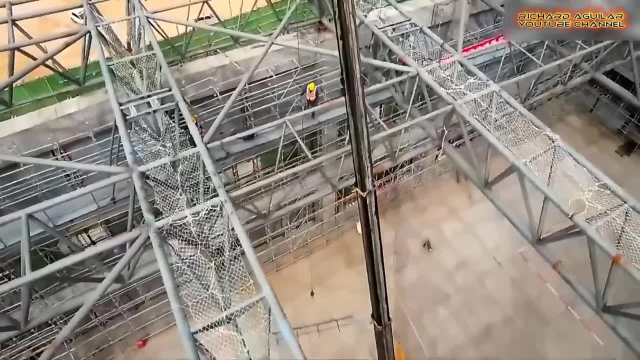 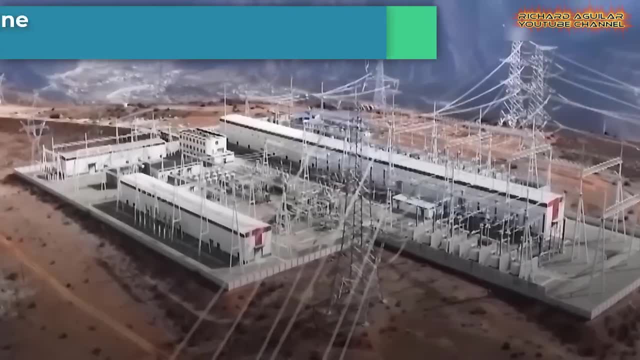 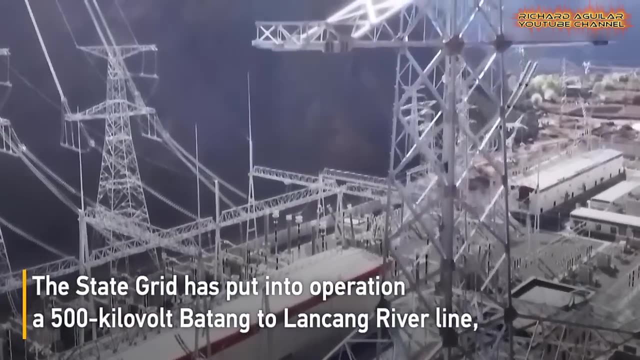 The station is expected to play a crucial role in improving transportation connectivity and promoting economic development in the region. China's state grid has put into operation a 500-kilovolt Badong-to-Longtsong River line, adding another 500-kilovolt transmission line between southwest China's Sichuan and Tibet. 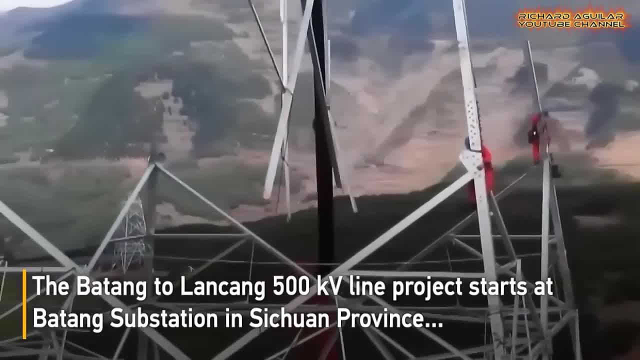 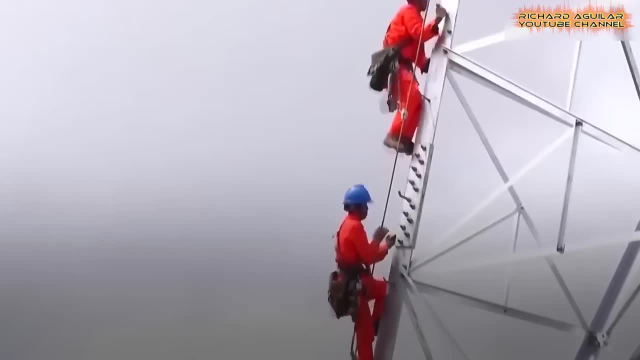 The 500-kV line project starts at Badong substation in Sichuan Province and ends at Longtsong River substation in Tibet. The station is expected to be completed by the end of this year. Once it's operational, the power grids of the two regions will be able to support each other. 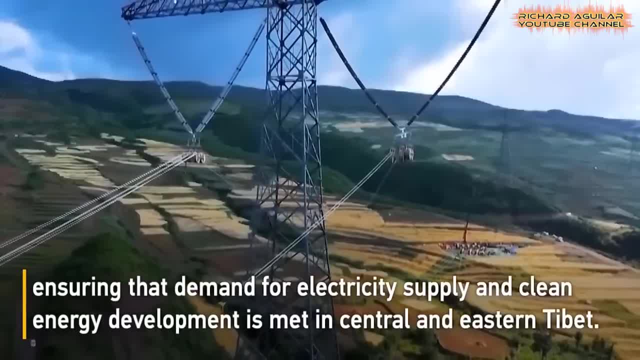 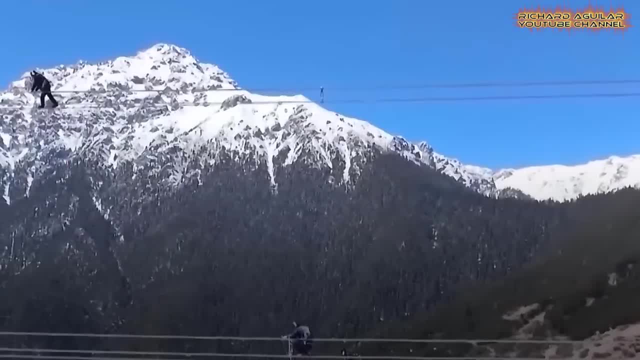 The power grids of the two regions will be able to support each other. Thank you for joining us for today's story. If you enjoyed this video, please give us a thumbs up and share it with others. We appreciate your support and hope you have a fantastic day. 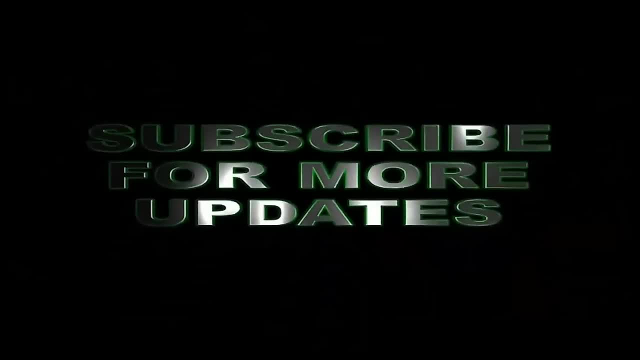 If you have any questions or other problems, please post them in the comments below.